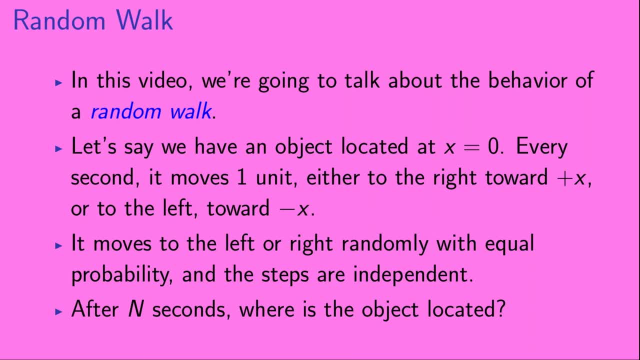 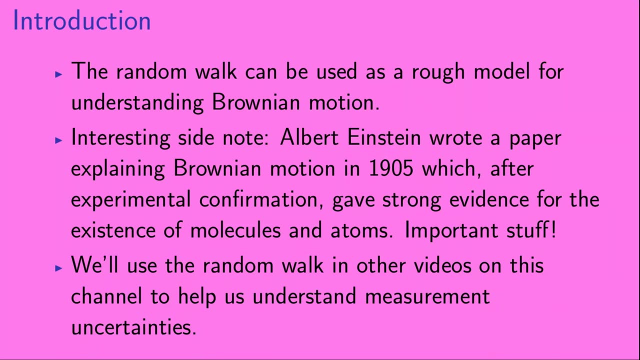 x. It moves to the left or right randomly with equal probability and the steps are independent After n seconds. where is the object located? The random walk can be used as a rough model for understanding Brownian motion. Here's an interesting side note: Albert Einstein wrote a paper explaining Brownian motion in. 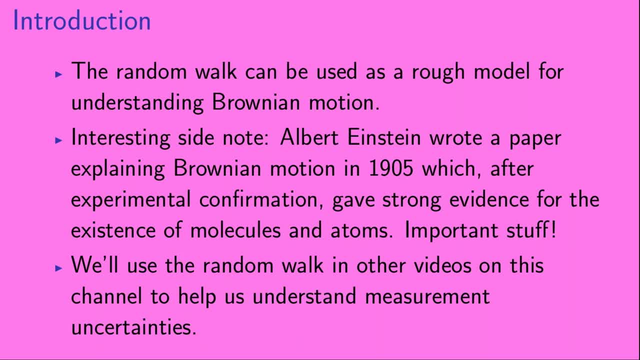 1905, which, after experimental confirmation, gave strong evidence for the existence of molecules and atoms. So that was important stuff. We'll use the random walk to explain Brownian motion in the future. Thank you for watching and I'll see you next time. 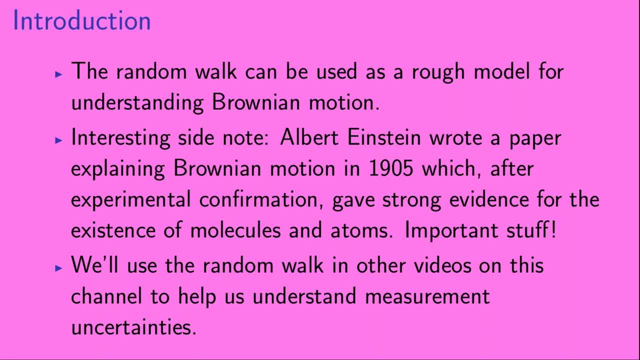 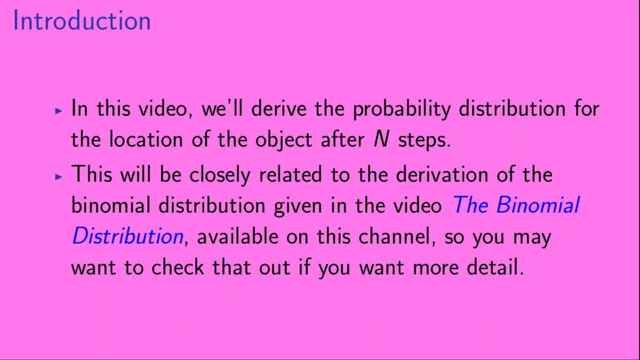 in other videos on this channel to help us understand measurement uncertainties. In this video we'll derive the probability distribution for the location of the object after n steps. This will be closely related to the derivation of the binomial distribution given in the video. the binomial distribution available on this channel. 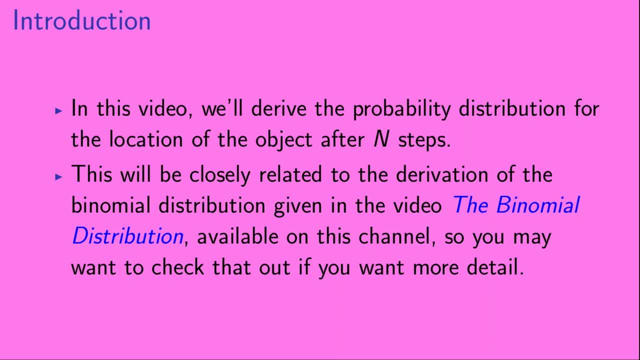 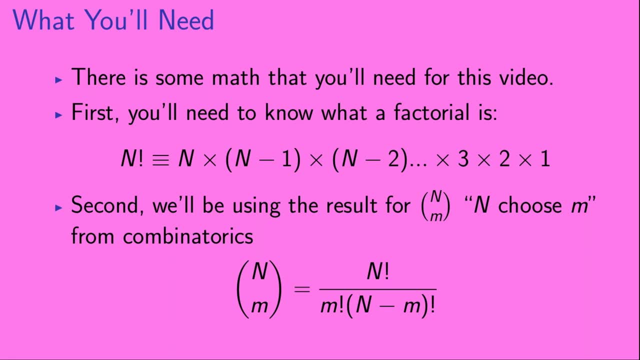 so you may want to check that out if you want more detail. Okay, so there is some math that you're going to need for this video. First, you'll need to know what a factorial is, So n factorial written as n with an exclamation. 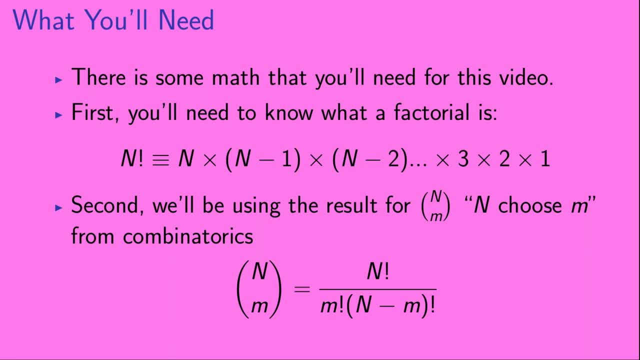 point after, it is defined to be n times n minus 1 times n minus 2, etc. all the way down to 1.. Second, we'll be using the result for n. choose m from combinatorics, which is equal to n factorial. 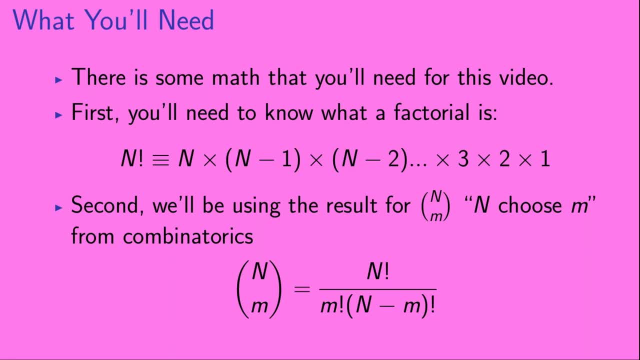 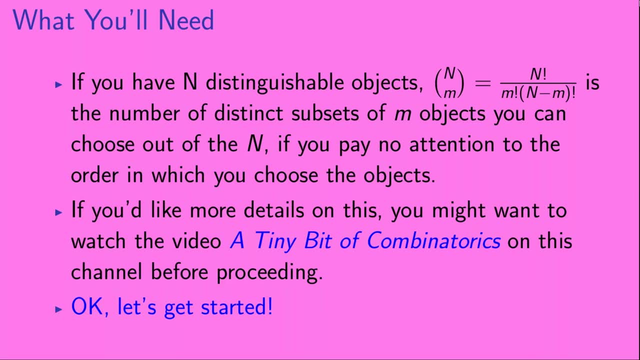 over m factorial. n minus m factorial. So if you have n distinguishable objects, n choose. m is the number of distinct subsets of m objects. you can choose out of the n if you pay no attention to the order in which you choose the objects. If you'd like more details on this, you might want to check out the video, A Tiny Bit of. 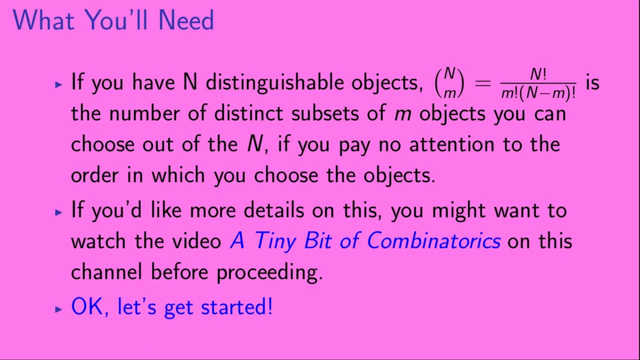 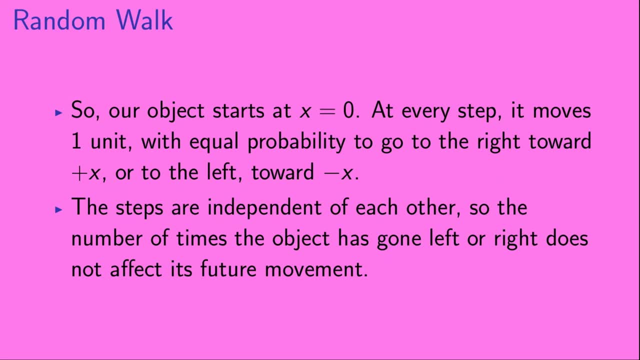 Combinatorics on this channel before proceeding. Okay, let's get started. So our object starts at x equals zero. At every step it moves one unit, with equal probability to go to the right toward plus x, or to the left toward minus x. The steps are independent of each. 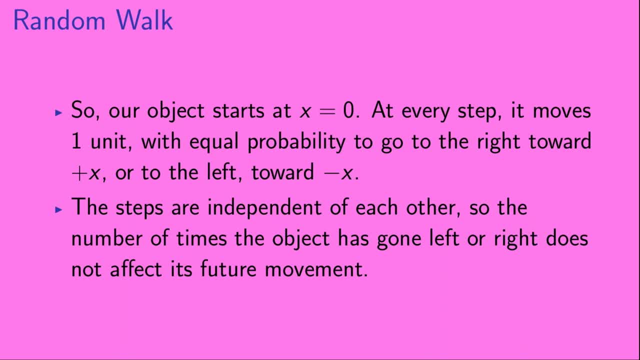 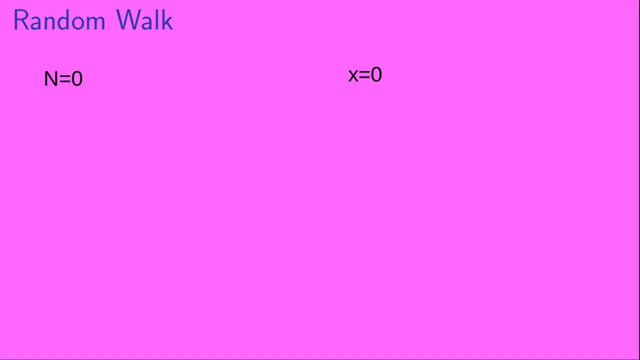 other. so the number of times the object has gone left or right does not affect its future movement. So the object starts at x equals zero. After one step it can be at x equals minus one or at x equals one. After two steps it can be at x equals minus two, at x equals zero or at x equals two. 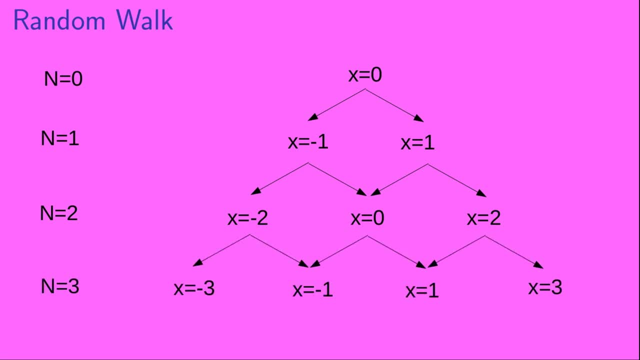 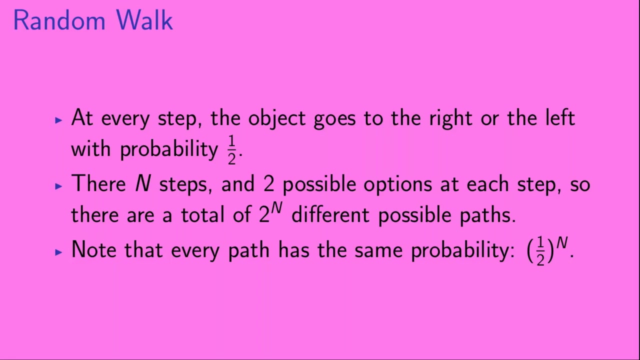 And after three steps it can be at x equals minus three, x equals minus one, x equals one or x equals three. At every step the object goes to the right or the left, with probability one half. There are n steps and two possible options at each step, so there are a total of two to the n. 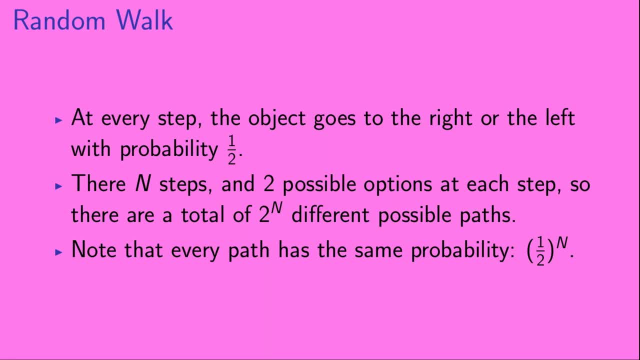 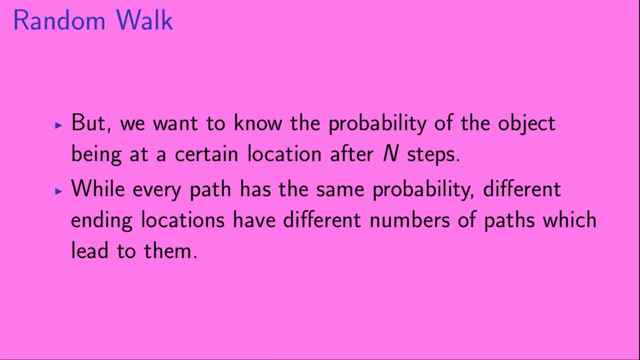 different possible paths And note that every path has the same probability- one half raised to the n power probability of the object being at a certain location after n steps. While every path has the same probability, different ending locations have different numbers of paths which lead to them. So, for example, for n equals 2, there 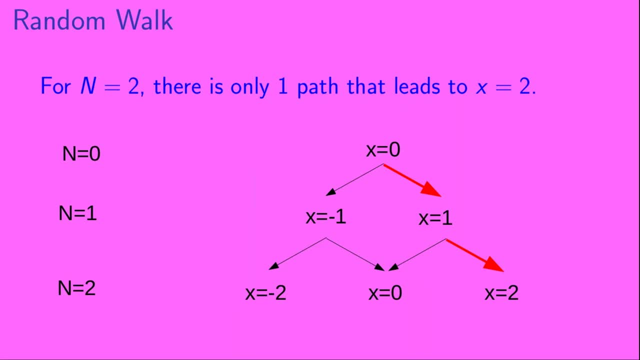 is only one path that leads to x equals 2.. And, similarly, there is only one path that leads to x equals minus 2.. However, there are two paths that lead to x equals 0.. The object can go to the right and then to the left, or it can go to the. 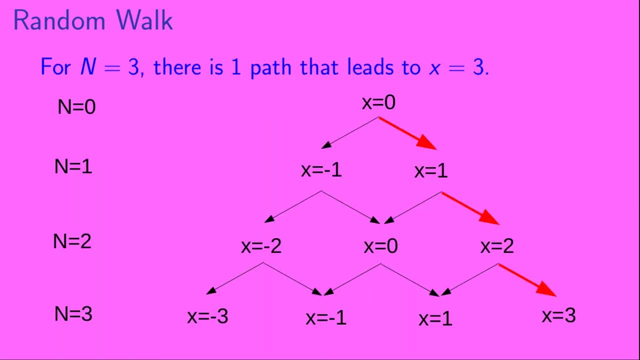 left and then to the right. For n equals 3, there is one path that leads to x equals 3.. However, there are three paths that lead to x equals 1.. So the object can go to the right, to the right and then to 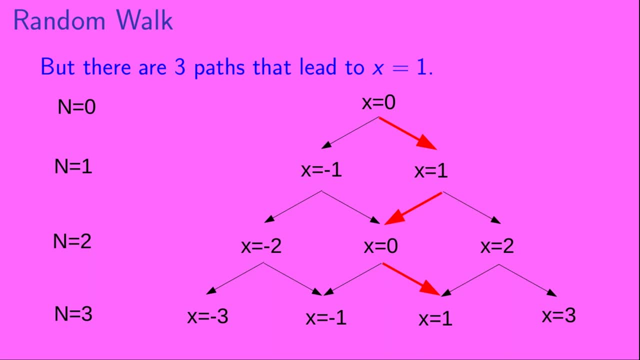 the left or to the right, then to the left and then to the right, Or it can go to the left, then to the right, then to the right. For all three of those paths the object ends up at x equals 1.. So all paths are equally likely, but we need to 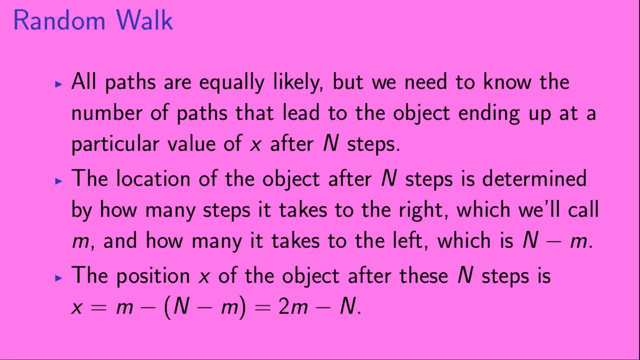 know the number of paths that lead to the object ending up at a particular value of x after n steps. The location of the object after n steps is determined by how many steps it takes to the right, which we'll call m, and how many it takes to the left, which would be n-m. 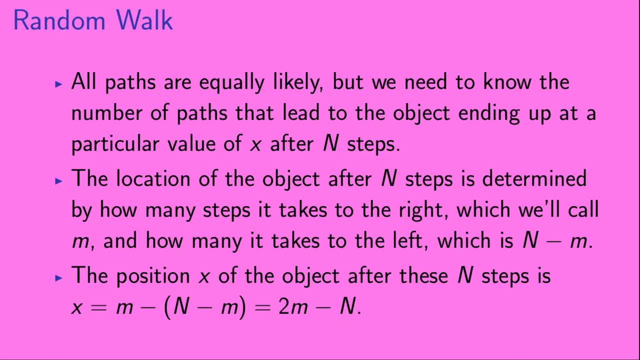 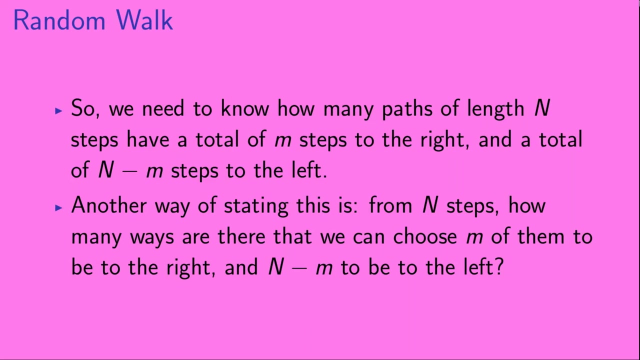 The position x of the object after these n steps is: x equals the number of steps to the right, which equals m, minus the number of steps to the left, which equals n-m. So that gives x equals 2m-n. So we need to know how many paths of length n steps have a total of m steps to the right. 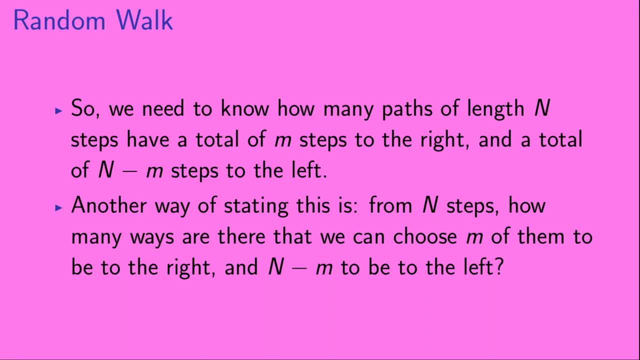 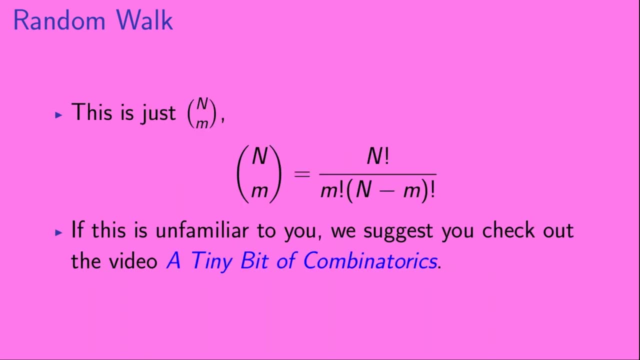 and a total of n-m steps to the left. Another way of stating this is: from n steps. how many ways are there that we can choose m of them to be to the right and n-m of them to be to the left? 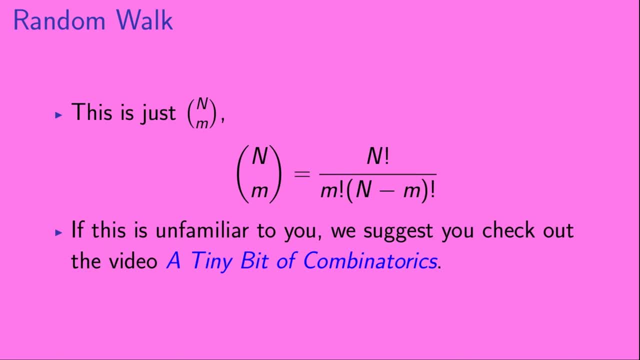 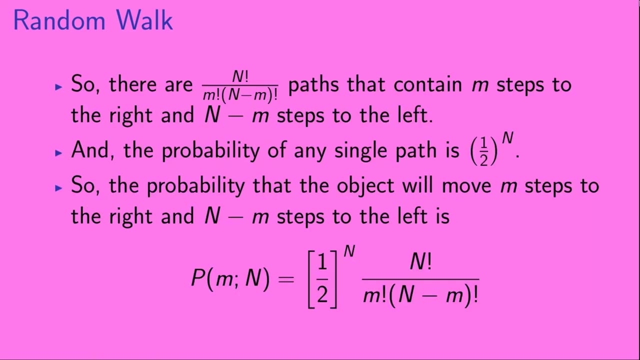 Now this is just n choose m, which, as we said before, is equal to n factorial over m factorial, n minus m factorial. If this is unfamiliar to you, we suggest you check out the video. A Tiny Bit of Combinatorics. 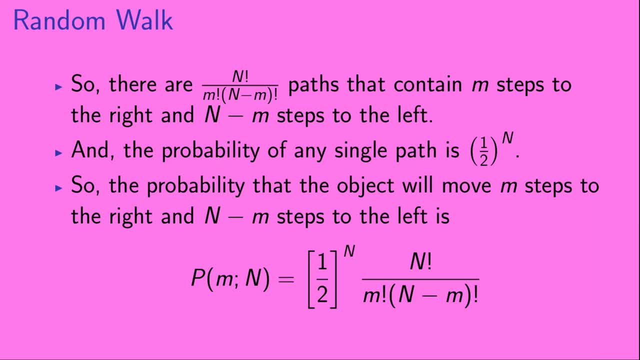 So there are n factorial, n factorial Over m factorial, n minus m factorial牌θ that contain m steps to the right and n minus m steps to the left, And the probability of any single path is 1 half to the n-power. 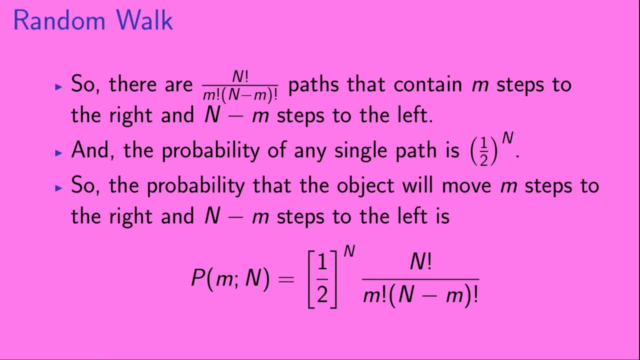 So the probability that the object will move m steps to the right and n minus m steps to the left is something that we are going to call p of m. given n, which equals 1 half raised to the n power, n factorial over m factorial, n minus m factorial. 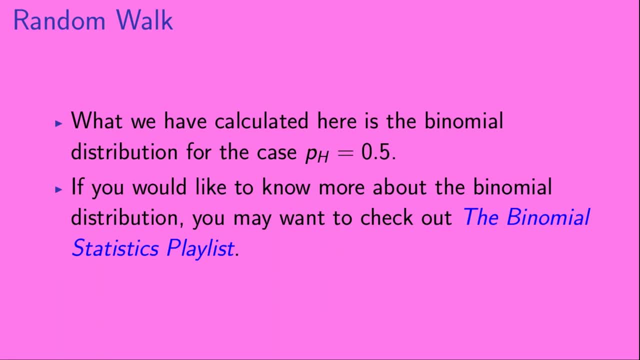 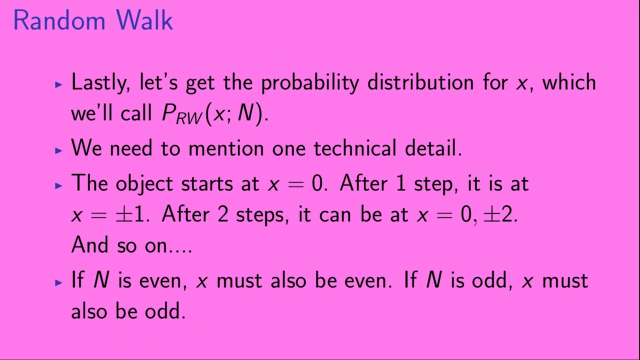 What we have calculated here is the binomial distribution for the case pH equals 0.5. If you would like to know more about the binomial distribution, you may want to check out the Binomial Statistics playlist on this channel. Lastly, let's get the probability distribution for x, which we'll call p, with a subscript rw of x given n. 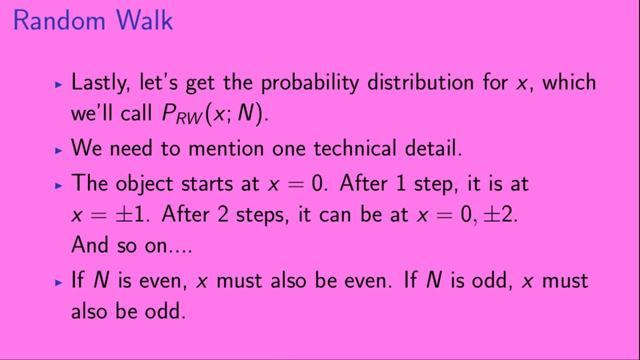 We need to mention one technical detail. The object starts at x equals 0.. After one step, it is at x equals plus or minus 1.. After two steps, it can be at x equals 0, or at plus or minus 2, and so on. 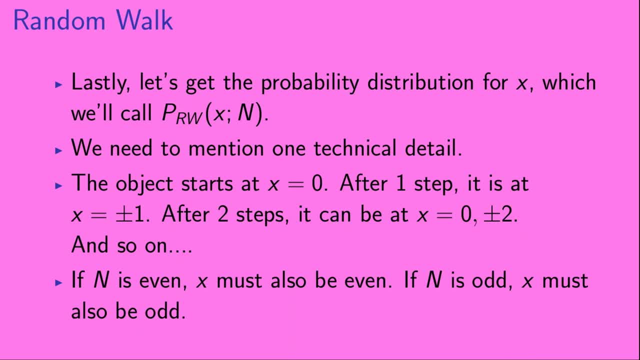 If n is 0,, it is at x equals 0.. If n is 0,, it is at x equals 0.. If n is even, x must also be even, And if n is odd, x must also be odd. 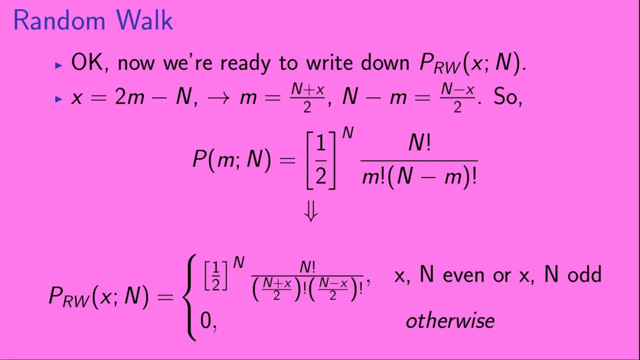 Okay, so now we're ready to write down our probability distribution for x. First we need to get m and n minus m in terms of x. So x is equal to 2m minus n, and this gives us that m is equal to. 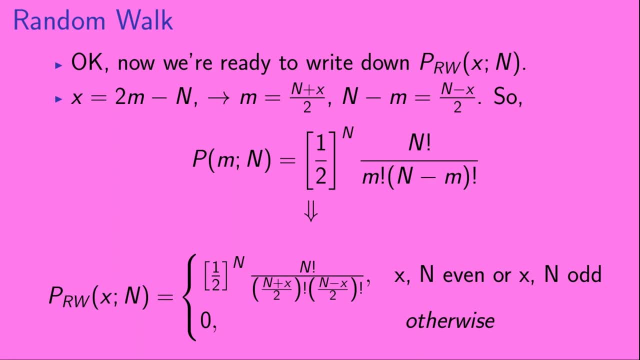 n plus x over 2, and n minus m is equal to n minus x over 2.. So from our probability distribution for m- p of m given n, we can get our probability distribution for x- p? rw of x given n. 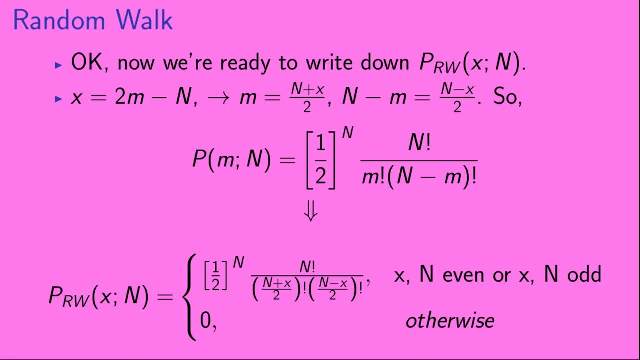 And our new probability distribution is equal to 1: half to the n times n. factorial over n plus x over 2, factorial n minus x over 2, factorial if x and n are both even or. 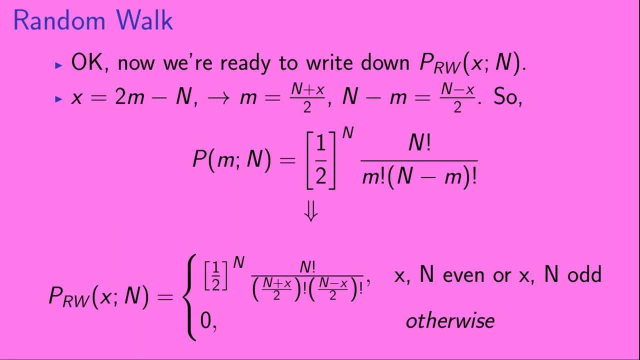 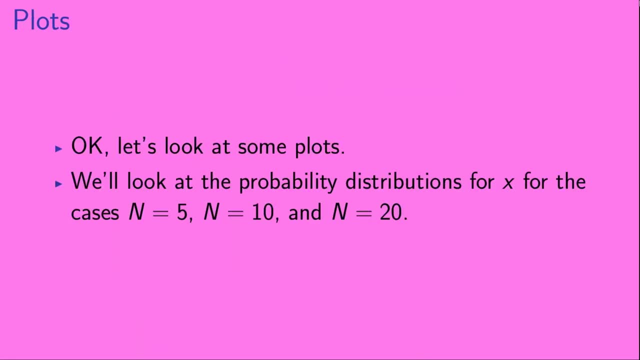 x and n are both odd And that's equal to 0,. if neither of those conditions is satisfied, Okay, let's look at some plots. We'll look at the probability distributions for x, for the cases n equals 5,. 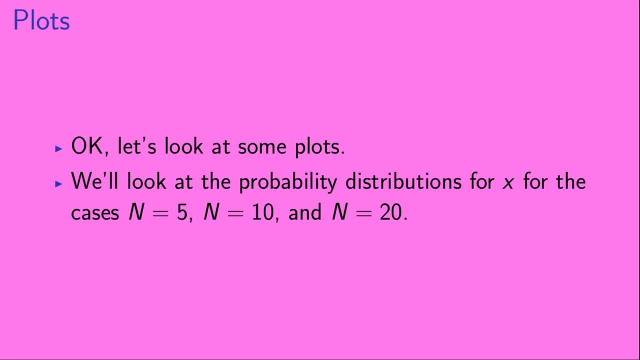 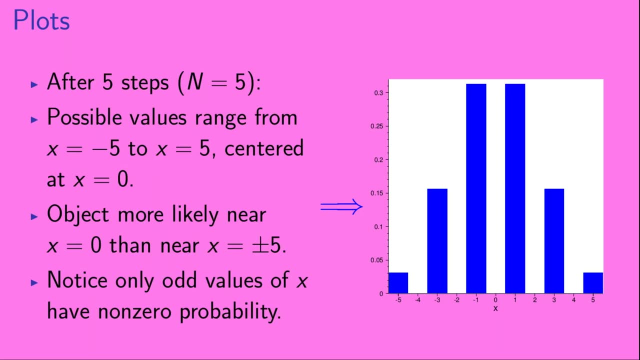 n equals 10, and n equals 20.. Okay, so first, after five steps. so n equals 5.. The possible values of x range from x equals minus 5, to x equals 5,, and the distribution is centered at x equals 0. 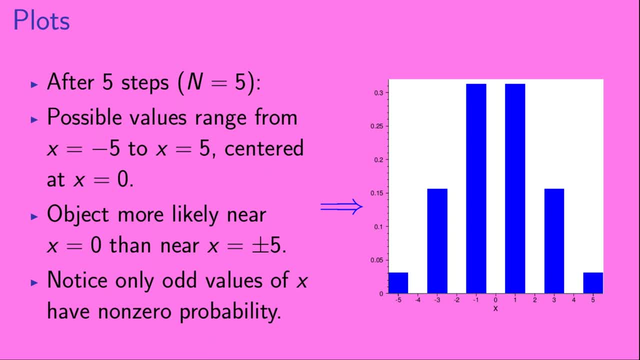 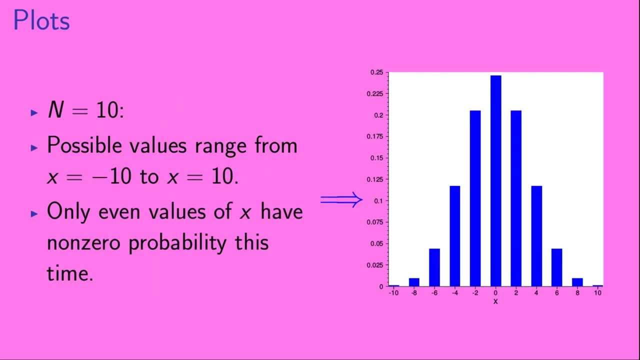 Notice that the object is much more likely to be near x equals 0, than near 0.. than near x equals plus or minus 5.. And only odd values of x have non-zero probability. Okay, next, n equals 10.. 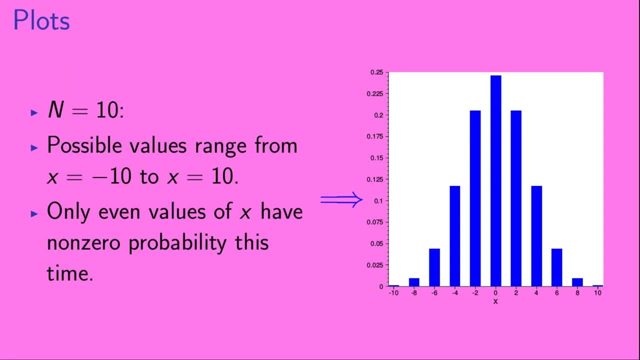 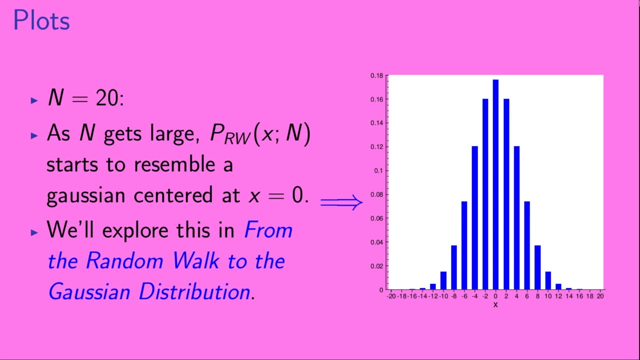 So here the possible values of x range from x equals minus 10, to x equals 10.. Only even values of x have non-zero probability this time. And lastly, here we display the probability distribution for n equals 20.. 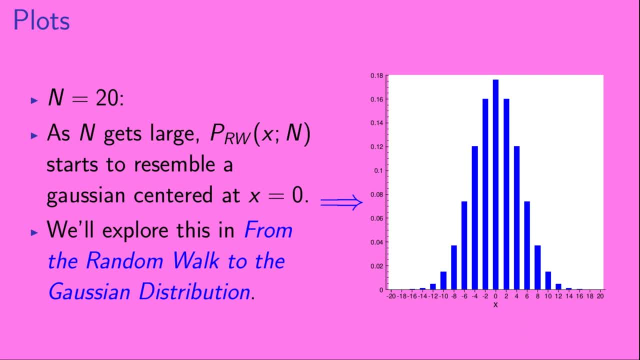 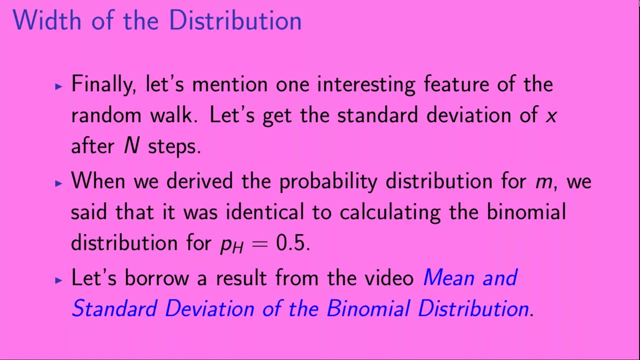 So as n gets large, the probability distribution for x starts to resemble a Gaussian centered at x equals 0. We'll explore this in From the Random Walk to the Gaussian Distribution. Okay, finally, let's mention one interesting feature of the random walk. 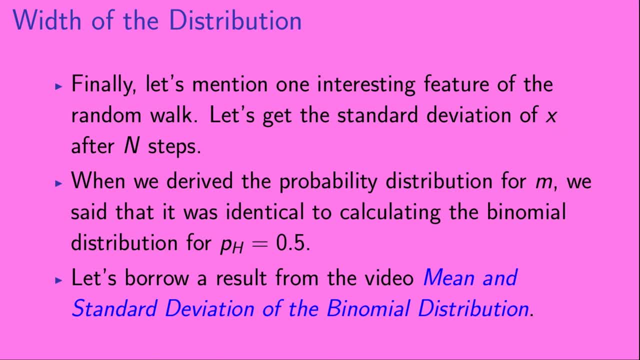 Let's get the standard deviation of x after n steps. When we derived the probability distribution for m, we said that it was identical to calculating the binomial distribution, for ph equals 0.5.. Let's borrow a result from the video. 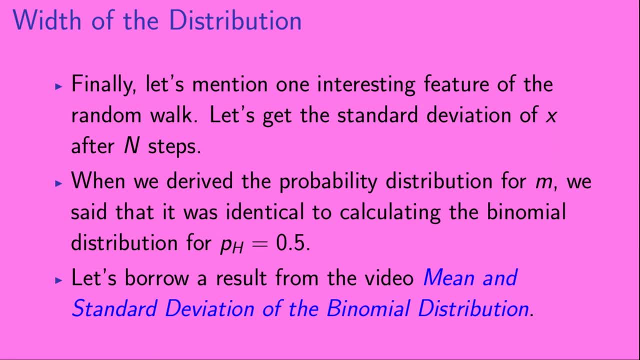 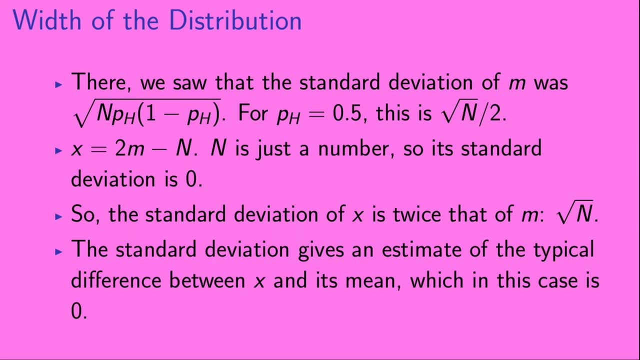 Mean and Standard Deviation of the Binomial Distribution. There we saw that the standard deviation of m was equal to the square root of n, ph 1 minus ph. For ph equal to 0.5, this is the square root of n. 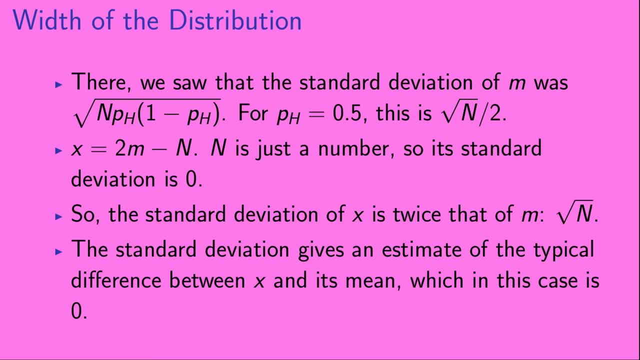 over 2.. Now x equals 2m minus n. n is just a number, so its standard deviation is 0.. So the standard deviation of x is just twice that of m. So the standard deviation of x. 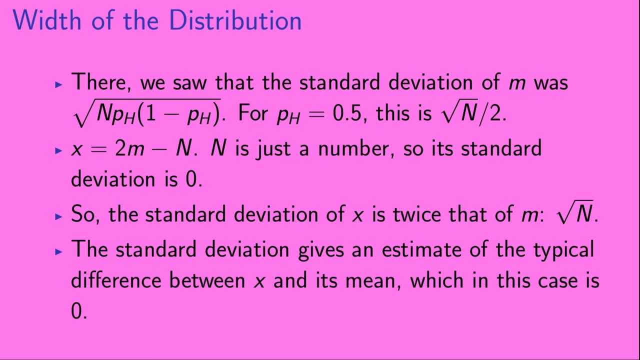 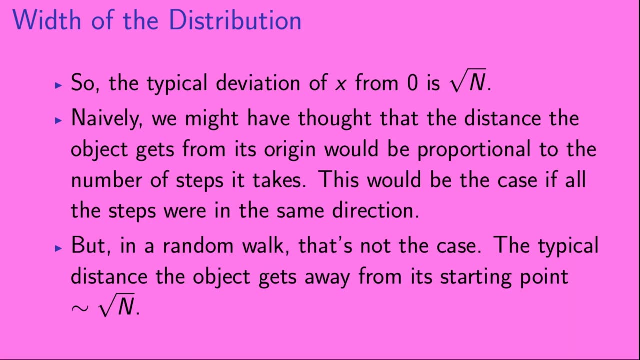 is equal to the square root of n. The standard deviation gives an estimate of the typical difference between x and its mean, which in this case is 0.. So the typical deviation of x from 0, is the square root of n. 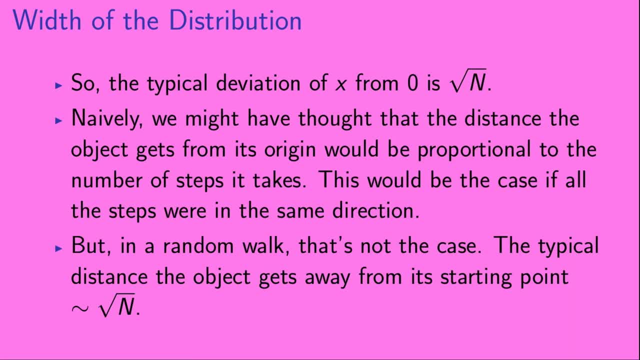 Naively, we might have thought that the distance the object gets from the origin would be proportional to the number of steps it takes. This would be the case if all the steps were in the same direction, But in a random walk. 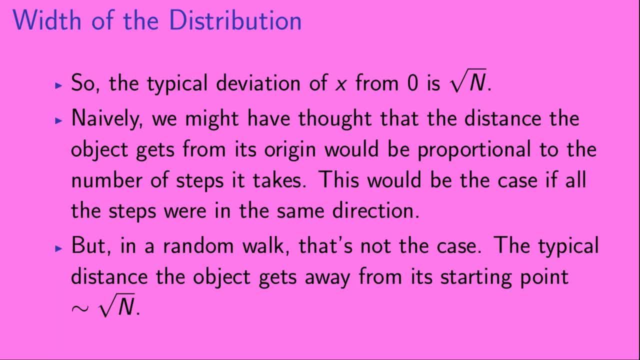 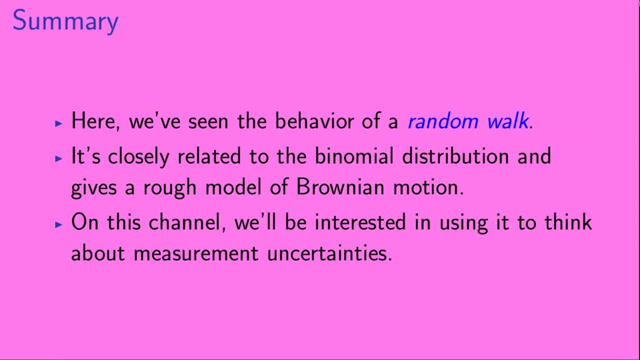 that's not the case. The typical distance the object gets away from its starting point goes as the square root of n. Okay, now let's summarize Here. we've seen the behavior of a random walk. It's closely related to the binomial distribution.